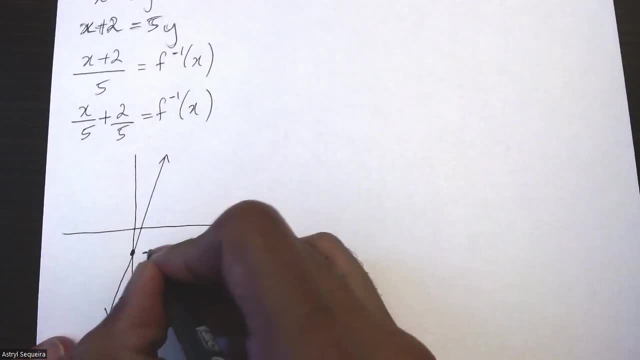 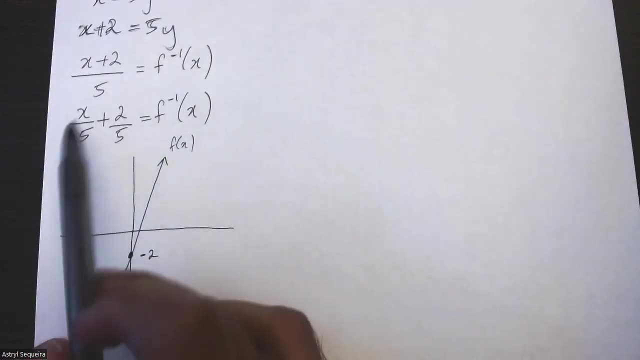 do a slope over here in the positive direction. That's the original function f of x. Now I want to sketch this out here, And this is why I split the denominator. I can tell that my y-intercept is 2 over 5. And my slope is positive, 1 over 5, which is positive but very flat. 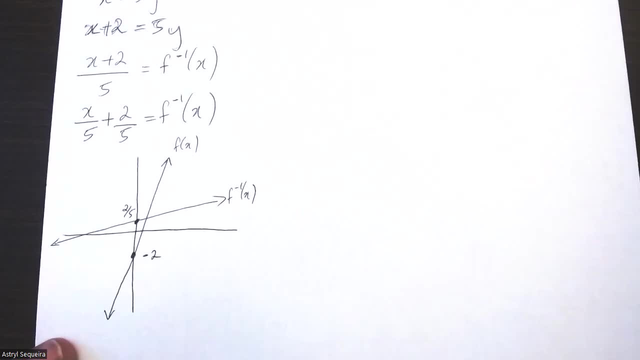 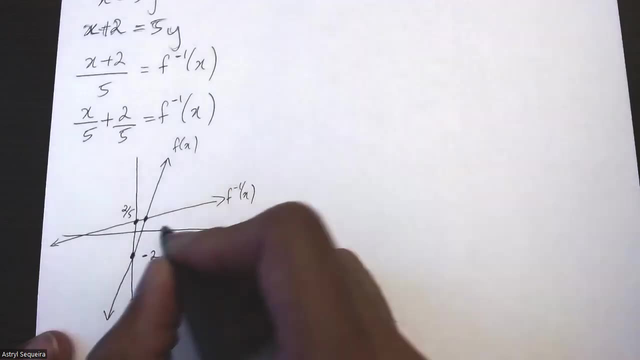 So that's a sketch of the inverse function. I can tell that these two functions intersect at a point over here And I want to find the x and y value of this point. So let's start by finding the x value. In order to find the x value of the point, you need to take the original. 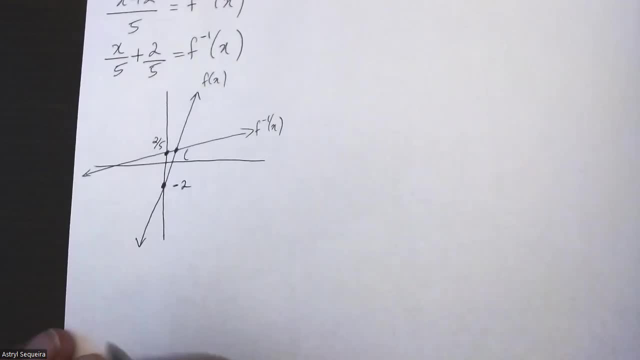 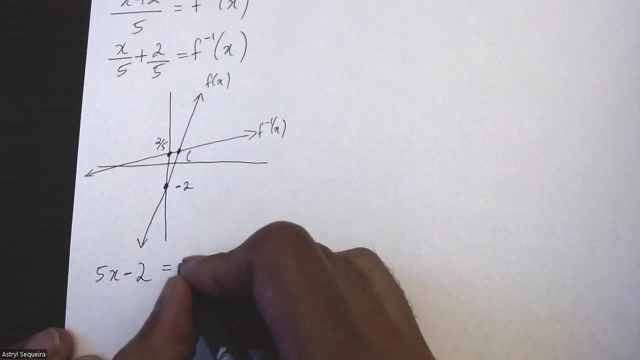 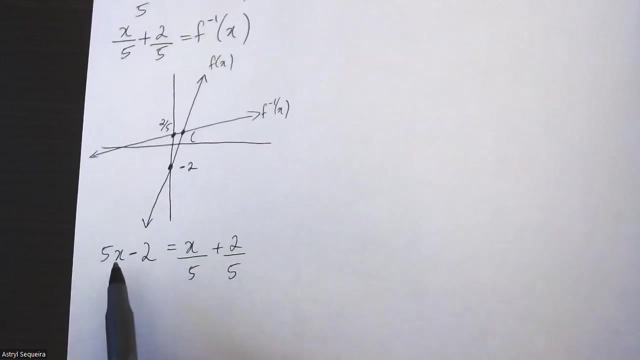 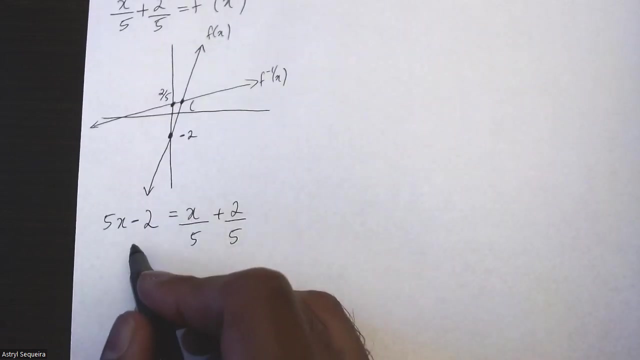 function and make it equal to the inverse function. So make the original equal to the inverse. Now we want to solve this. I'm going to start by moving this x over 5 to this side, And I'm going to move the negative 2 to the right side as well. 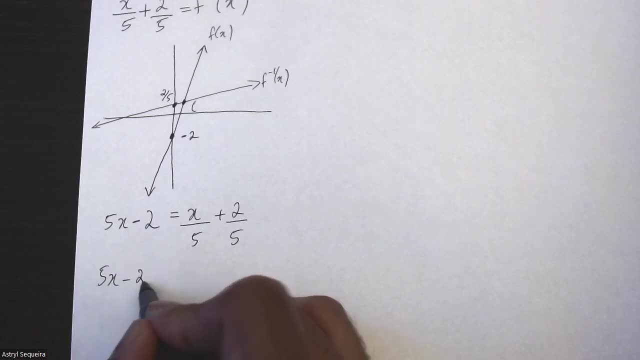 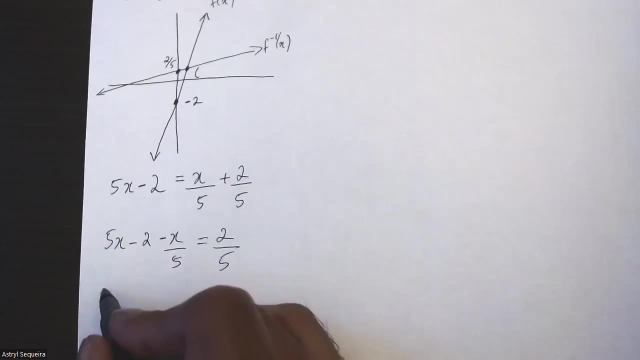 But I guess I 5x minus 2 minus x over 5 equals 2 over 5.. And I'll move the minus 2 to the other side. So you could do that in one step And that's how I'll do future questions. But I want to explain. 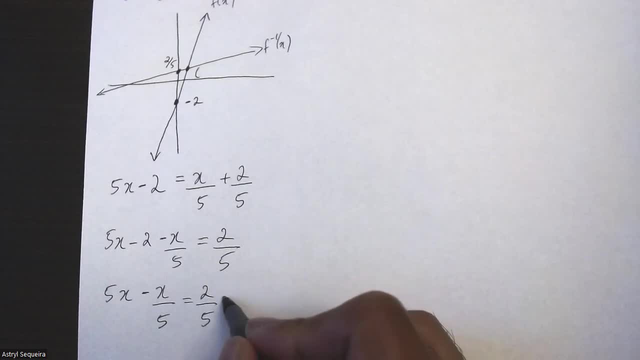 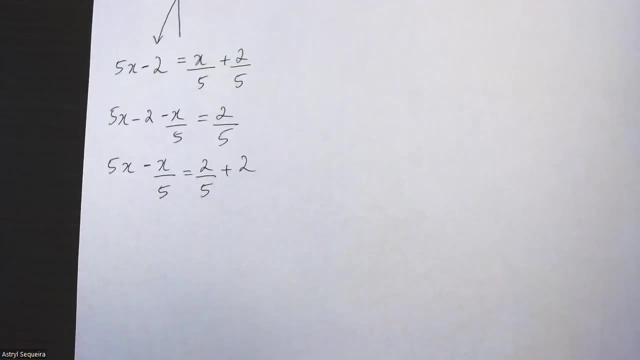 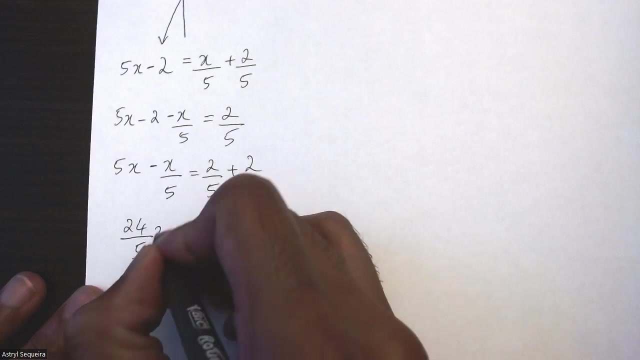 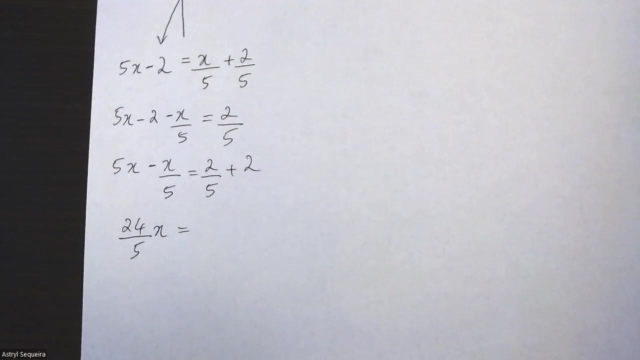 this a bit more clearly. So the negative 2 becomes a plus 2.. Now I just need to combine like terms. I'll do this in my calculator: 5 minus 1 over 5 is 24.. 4 over 5x, 2 over 5 plus 2 is 12 over 5.. And then I want to solve this. I have the same 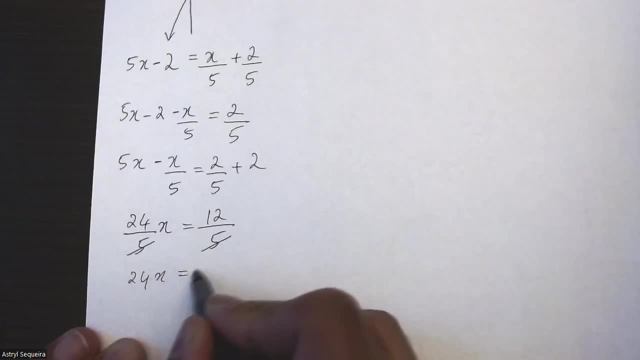 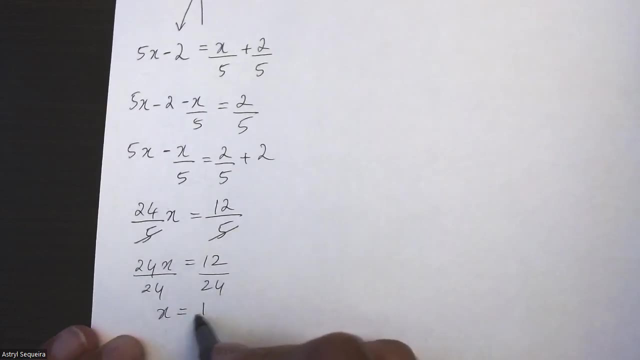 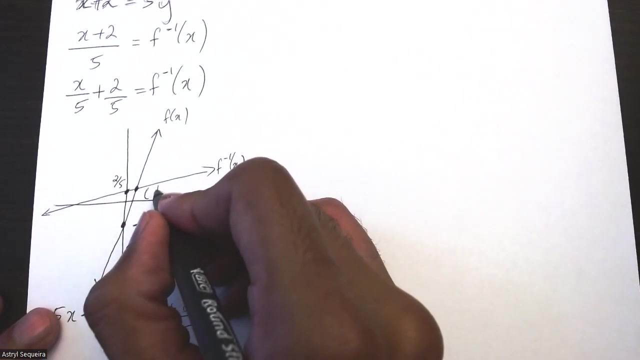 denominator. so I can cancel them. I just have 24x equals to 12.. And if I divide by 24 on both sides, I'll just get x equals 1 over 2. So this intersection point is 1 over 2.. To find the y value I just have to sub in 1 over 2. 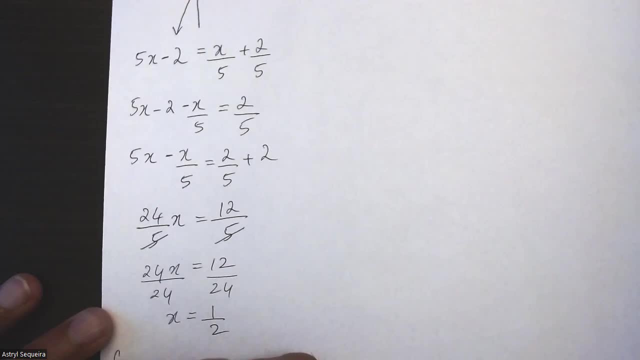 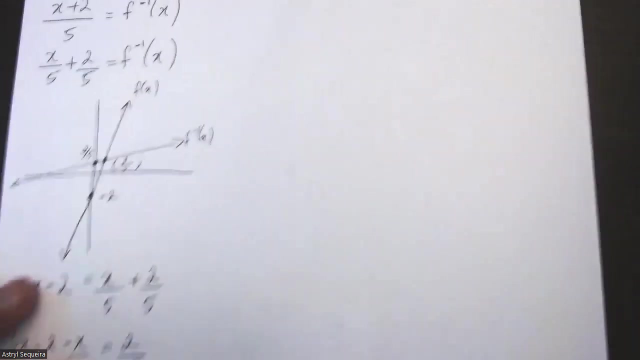 into the original function. So f of 1 over 2 is 5 times 1 over 2 minus 2.. Again, I'll do this in my calculator And I just get 1 over 2 as well, just by coincidence. So this intersection point. 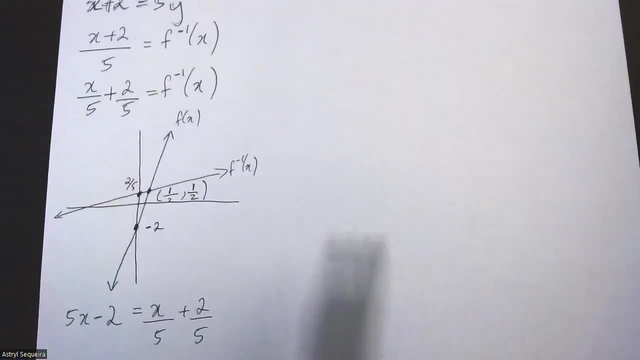 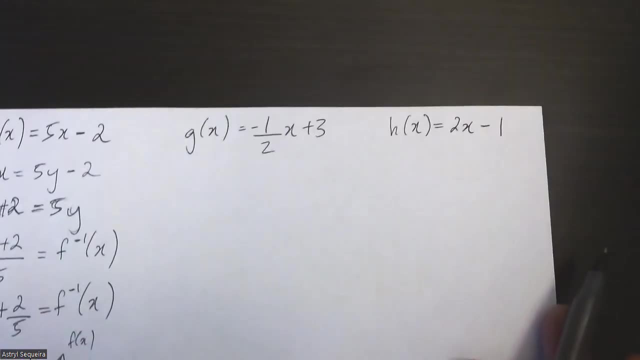 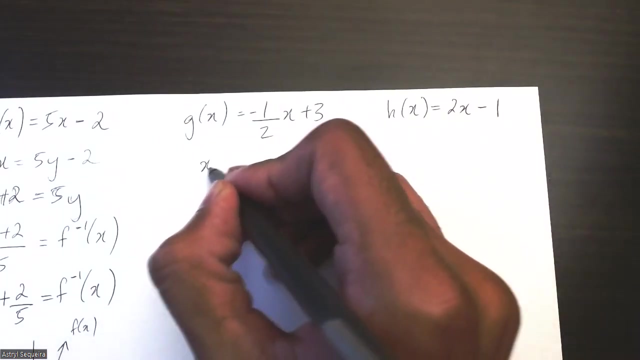 here. between these two functions, the original and its inverse is 1 over 2 and 1 over 2.. All right, So let's go to the next couple of examples. I'll solve these ones a bit quicker now that you know the steps. So let's start by finding the inverse. I'll switch my x and my y. 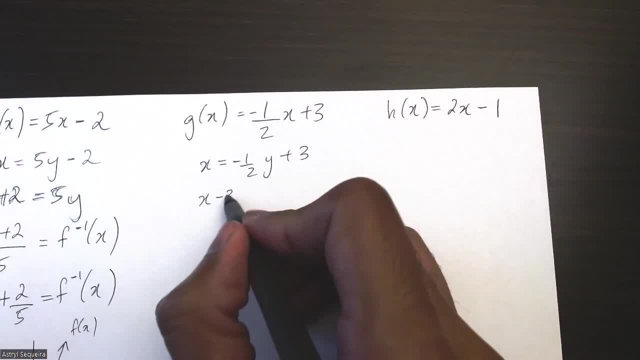 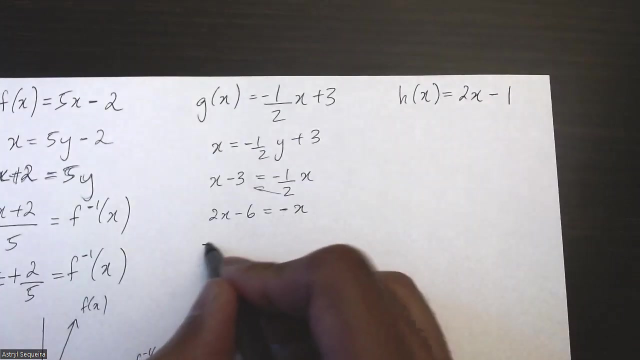 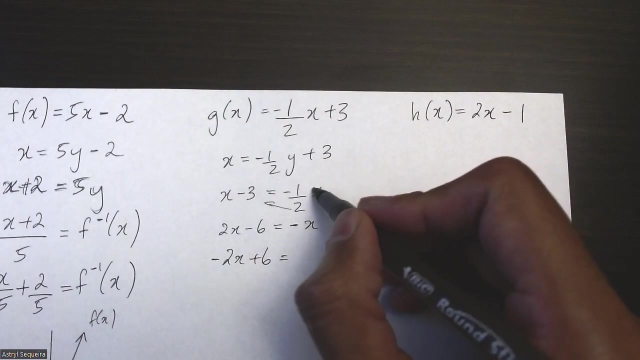 Then I'll isolate my y, I'll cross multiply this 2 over in the next step. So 2x minus 6 equals to negative x, And then I'll get rid of the negative by dividing everything by negative 1.. So this just becomes negative. 2x plus 6 equals- Oops, I don't know why I wrote an x here. 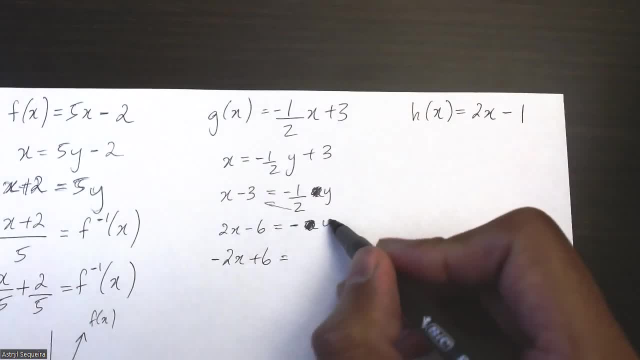 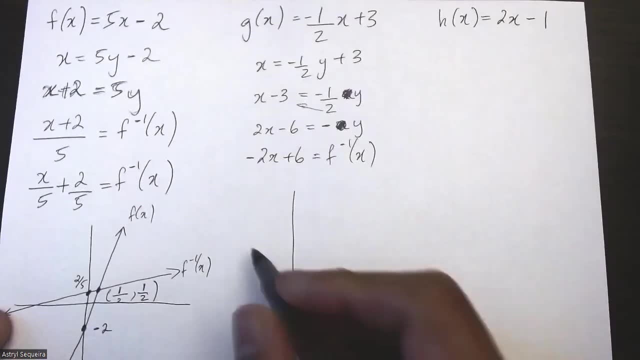 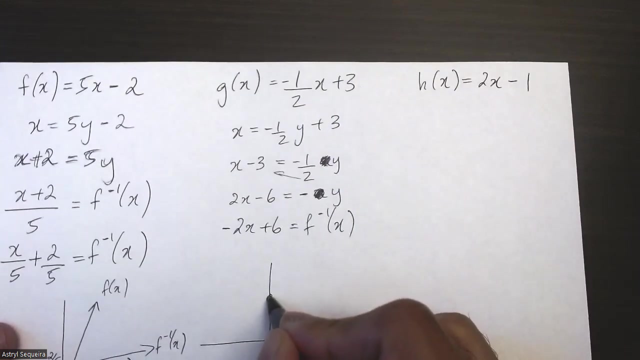 This is a y And then I write as f inverse of x. once it's isolated, I'll do my sketch next. So my first equation is negative 1 over 2x plus 3.. Y-intercept is 3. Slope is negative half. So negative slope, but not too steep. 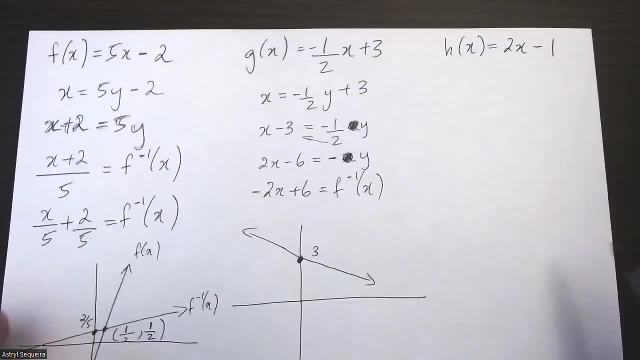 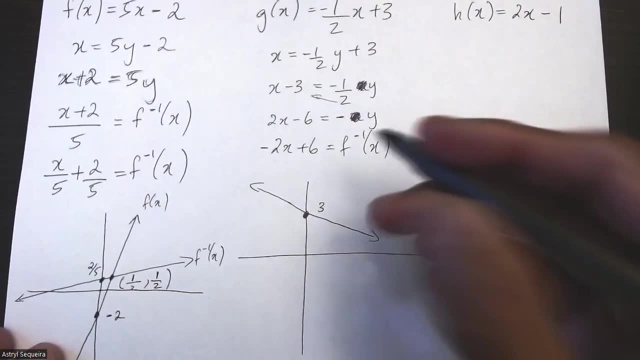 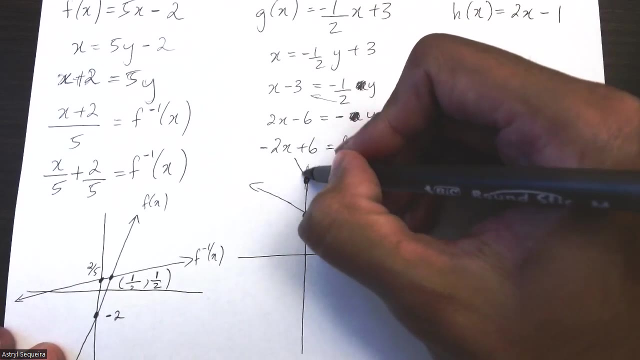 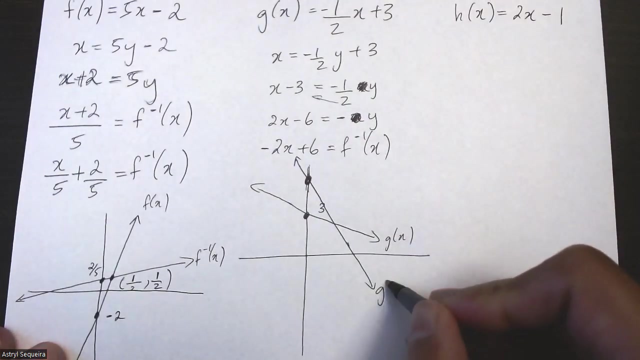 So it looks something like that Inverse equation has a y-intercept of 6. So slightly on top over here And it has a slope of negative 2. So negative slope, but a bit steeper, Just like that. That's g of x, That's g inverse of x And y-intercept is 6.. 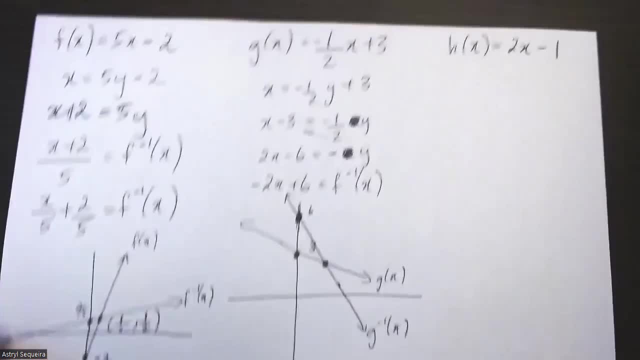 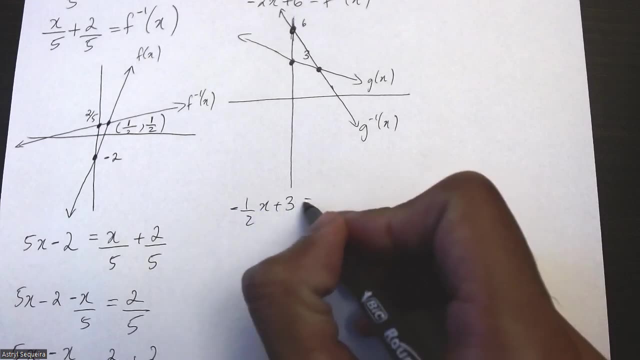 Now I need to find this point of intersection. I'm going to equate the original and the inverse with each other. Negative 1 over 2x plus 3 equals negative 2x plus 6.. I'll move this to this side. 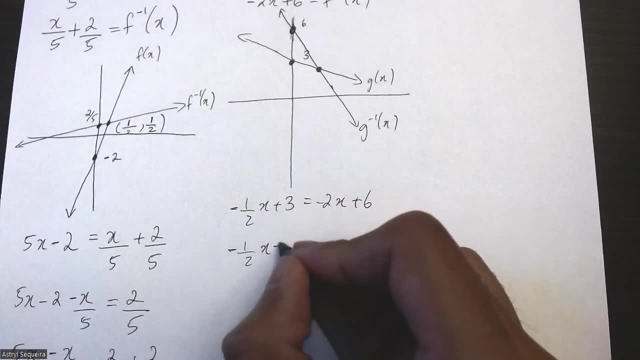 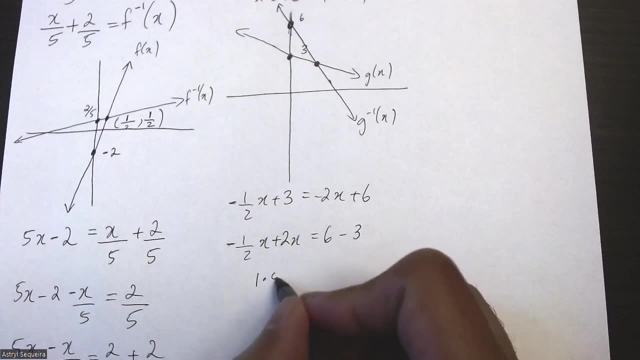 and the 3 to the other side. So negative: 1 over 2x plus 2x equals 6 minus 3.. That's just 1.5x or 3 over 2x, Doesn't matter which way you write it. 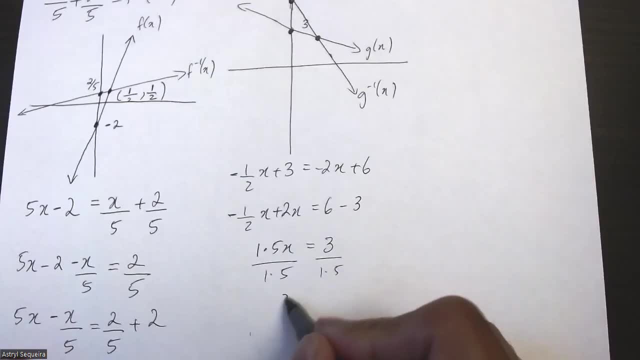 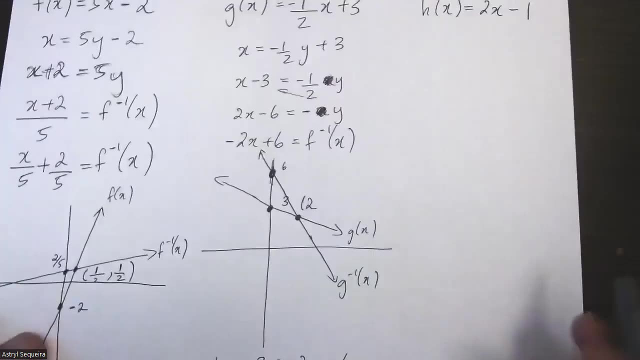 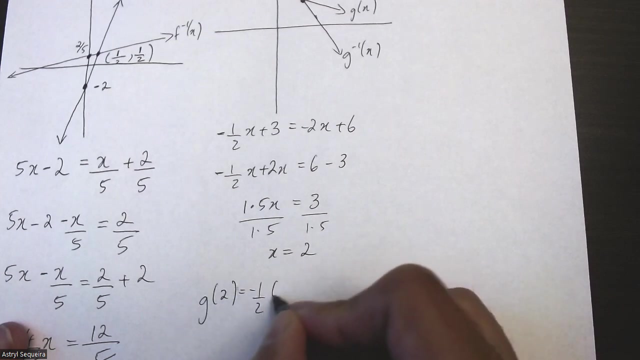 Now I'll divide by 1.5 on both sides, So I'll get x equals 2.. The x value of this point of intersection is 2.. Find the y value. I can solve it back into the original equation. So g of 2 equals negative 1 over 2 times 2 plus 3, which is just positive 2 again. 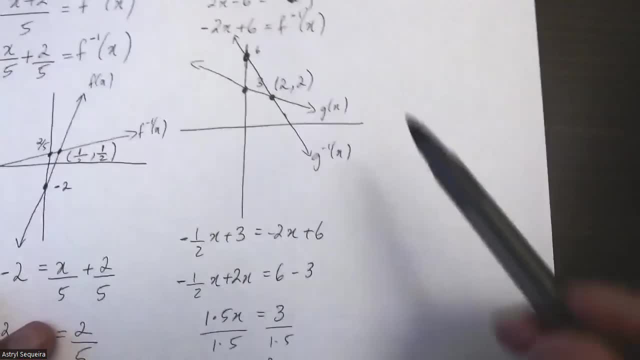 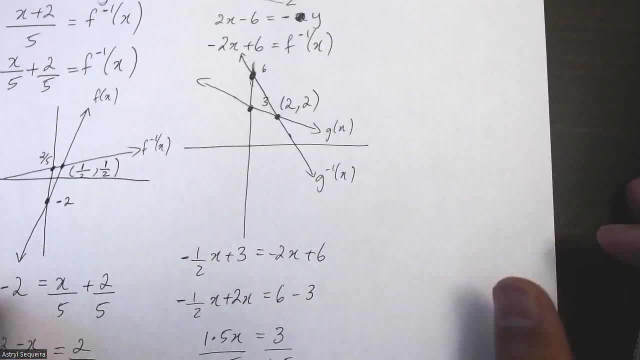 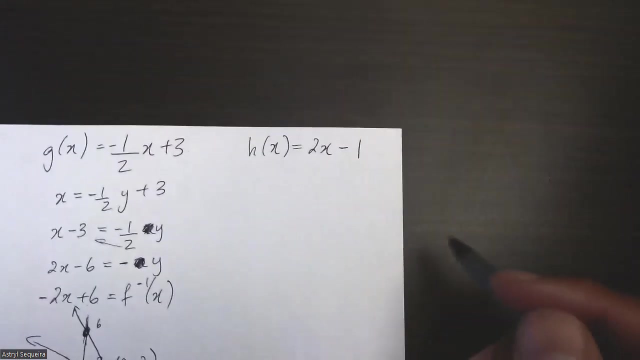 And we get the intersection point of 2. 2. It looks like x and y are the same in both cases. I wonder if that's true for all cases. It might actually be possible. Let's actually do all the examples and see if that actually works or not. Third one: here I want to find the inverse. So 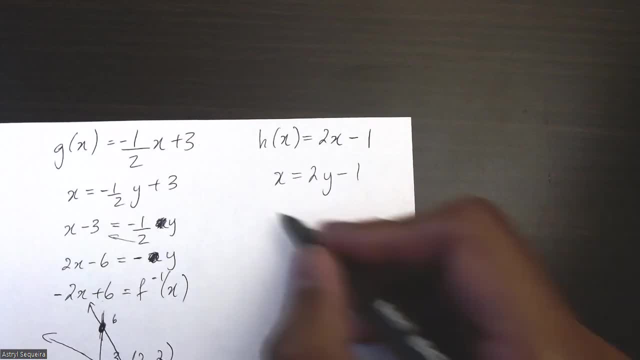 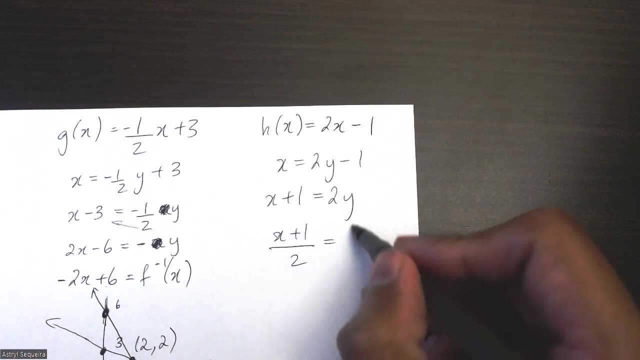 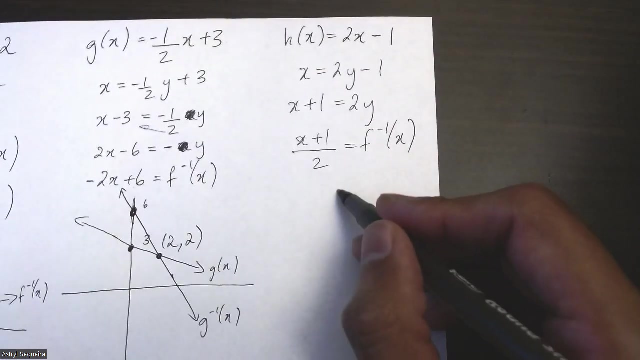 I'm going to flip my x and my y. I'm going to move the minus 1 to the other side. It becomes plus 1.. And then I'm going to divide by 2.. I get this. Now I want to sketch them both out. 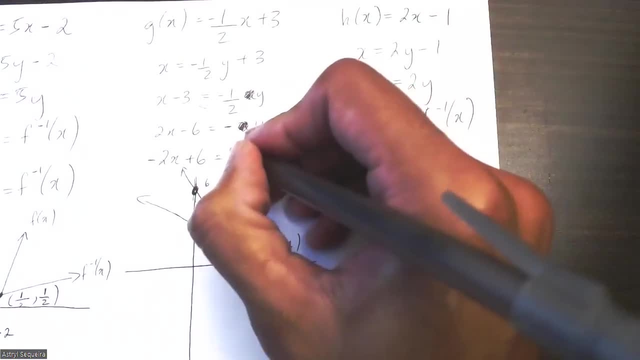 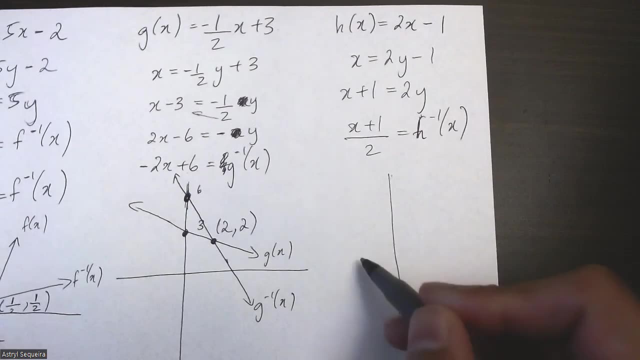 Also- this is sorry- h inverse of x And over here it should have been g inverse of x. I've labelled them wrong. It is g and then h over here. So if I do the graph, the slope is the y-intercept is negative 1 and slope is positive 2.. 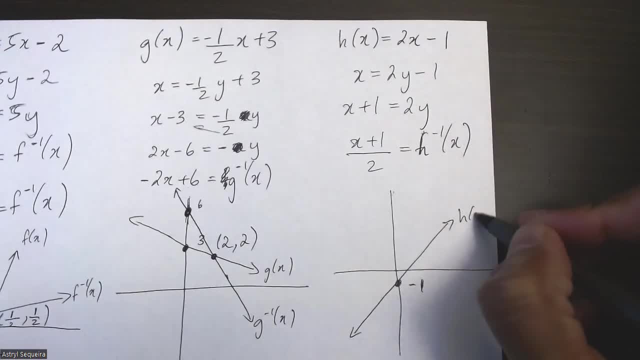 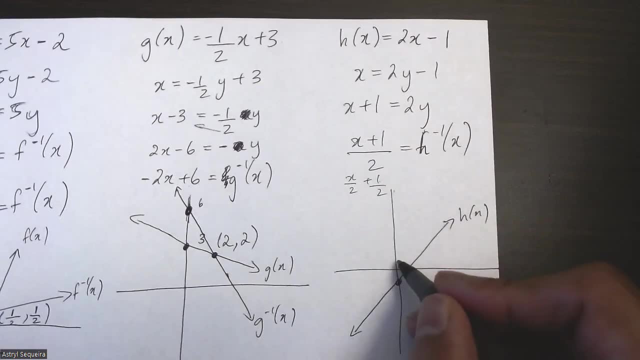 It looks like something like that: That's h and then the inverse. Again, you can split this into x over 2 plus 1 over 2 to make it easier to sketch. So the y-intercept is 1 over 2 and the slope is also 1 over 2, which means it's more flat, It looks. 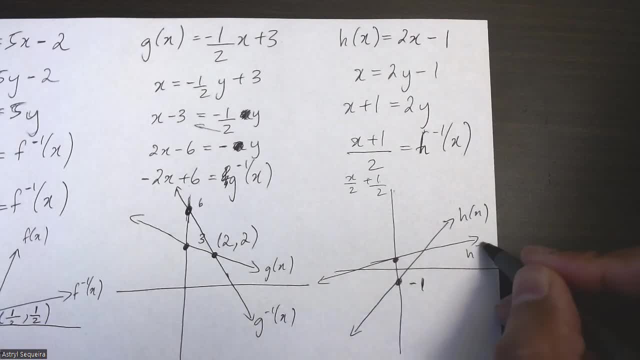 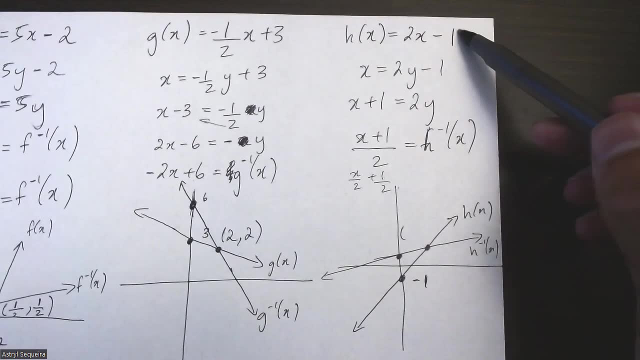 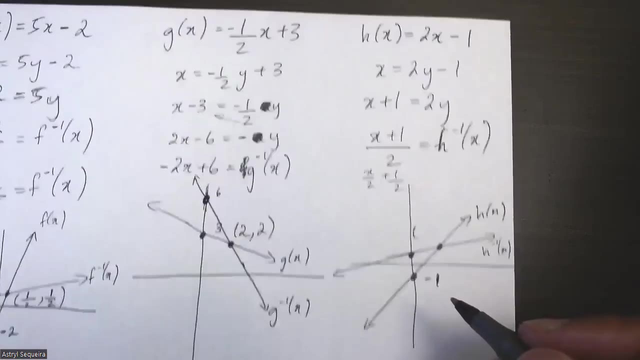 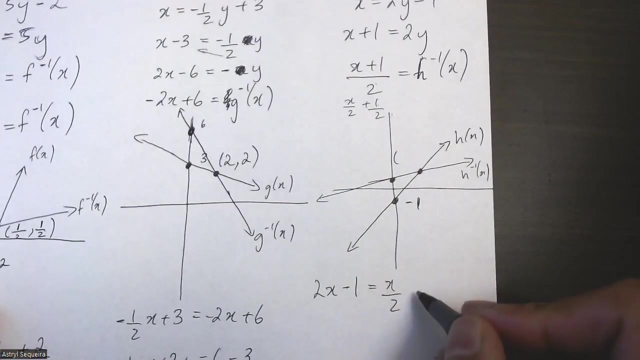 something like this: That's h inverse of x. The point of intersection is over here. I'll equate the original and the inverse to find the point of x-value of the point of intersection. So 2x-1 equals x over 2 plus 1 over 2.. I used a 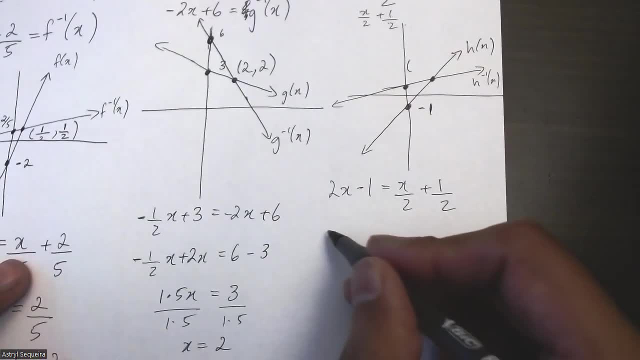 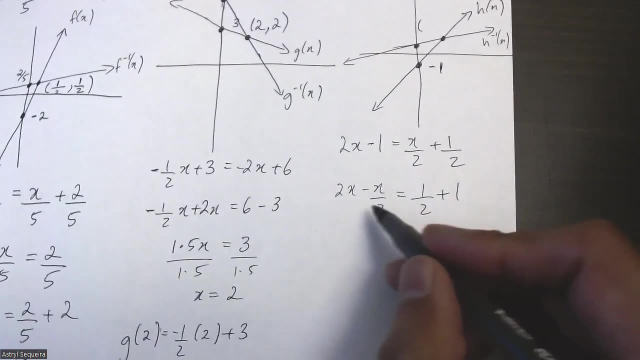 simplified one. I'll do a double movement here. So 2x minus x over 2 equals to 1 over 2 plus 1, and this is just again one- kayak. So 1.5 or 3 over 2x, whichever way you want to write it. i'll just write it as 1.5 because it's exact. 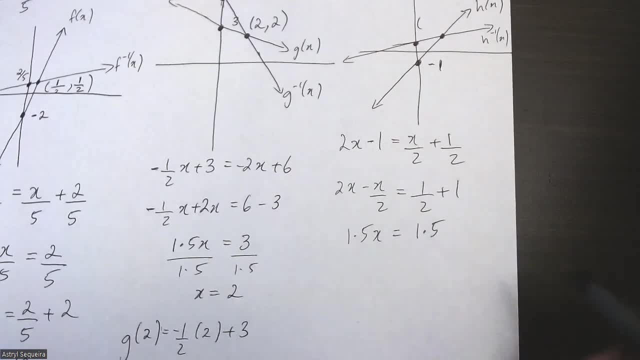 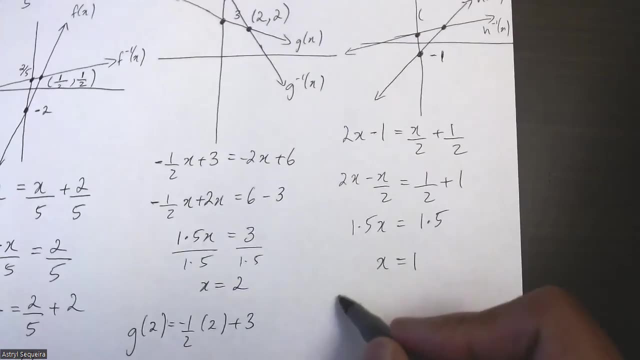 1 over 2 plus 1 is also 1.5. again, you could have used fractions there, which means x equals to 1 over here and i'll sub in this into the original equation. so h of 1 equals to 2 times 1 minus 1. 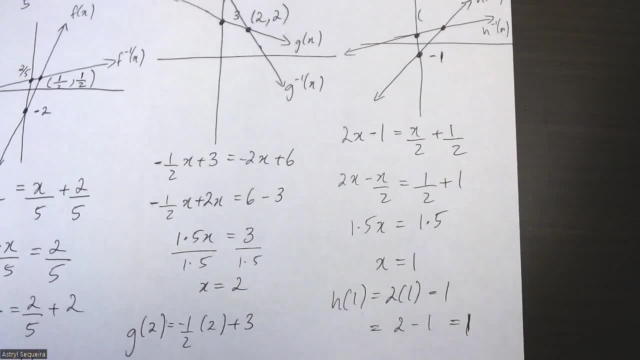 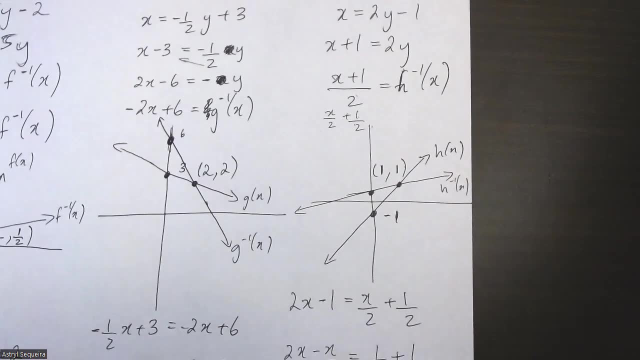 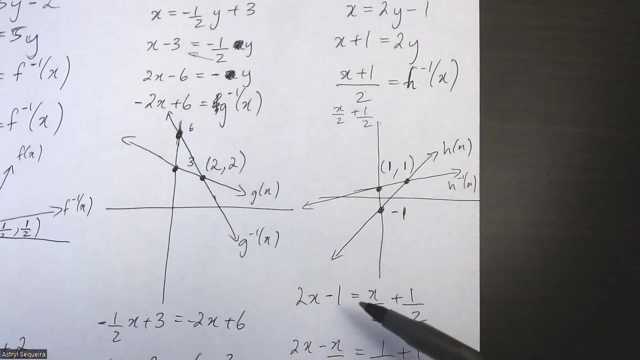 which is just 2 minus 1, which is also 1. so looks like every time we do this question the point of intersection x and y value are going to be the same, and i didn't know that was true, but i guess that's true for all inverse functions. if you have a function and you try to find the point, 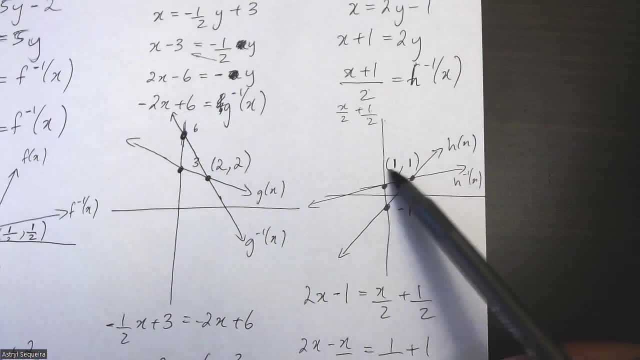 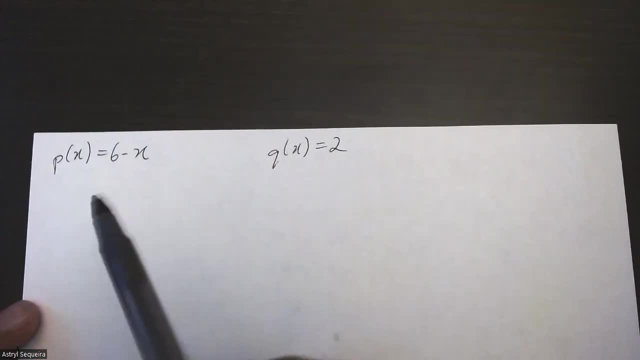 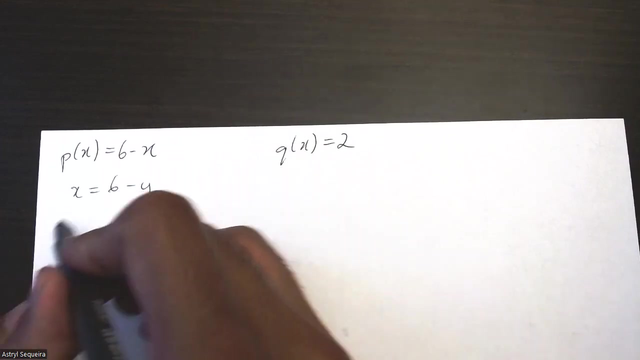 of intersection with its inverse. for linear functions at least x and y value will be the same. so even i learned something new this video, which is pretty cool. last two examples. i'll do them pretty quick. let's find the inverse over here. so x equals 6 minus y. 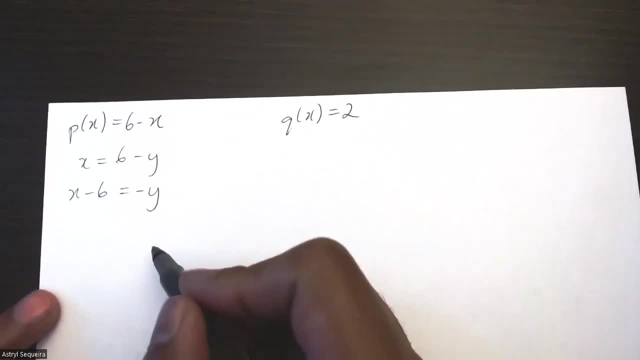 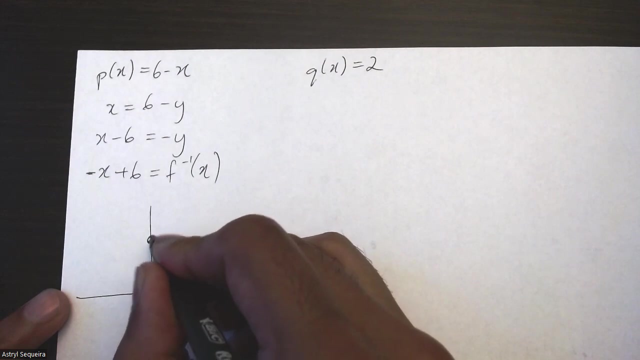 so x minus 6 equals minus y. i'll divide everything by negative 1. so negative x plus 6 equals f, inverse of x. plot these on my graph. so 6 minus x, i have a y-intercept of 6 and a slope of negative 1. 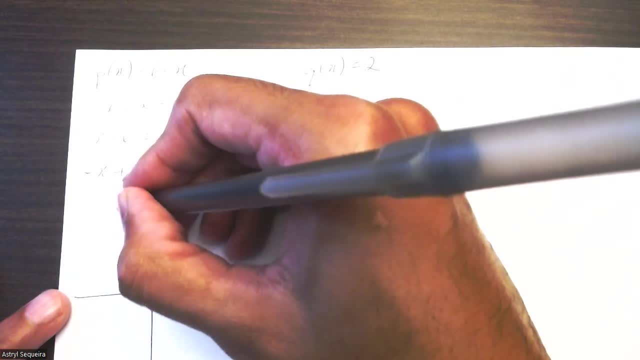 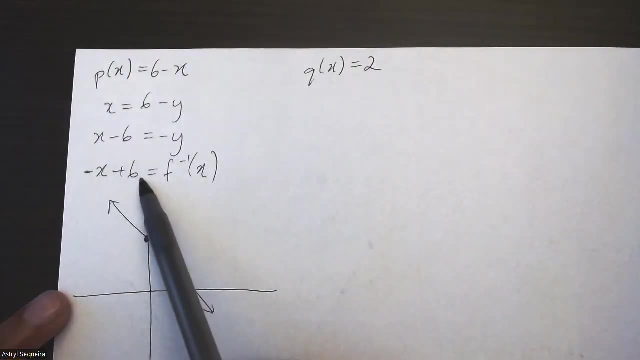 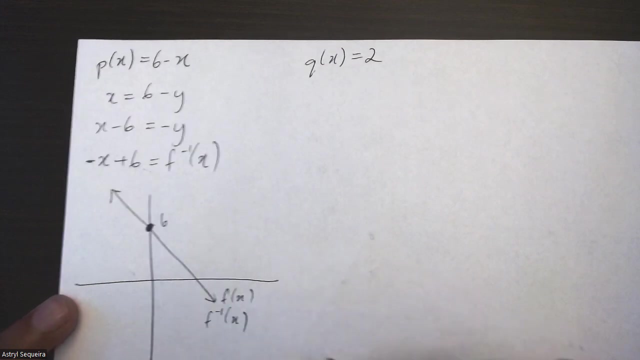 so it looks something like that: and negative x, x plus 6 is a y-intercept of 6 and a slope of negative 1, which is directly on top of this as well. so both lines- this is both f of x and f inverse of x, if both lines are top- are directly.